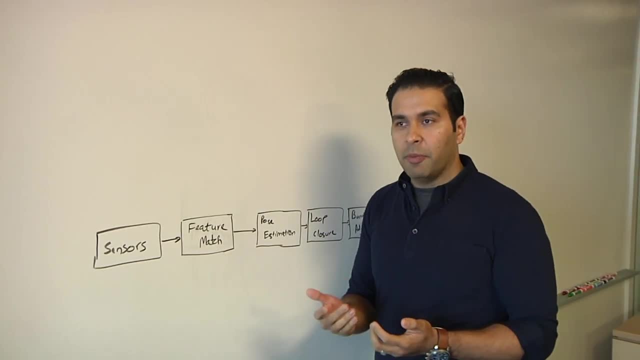 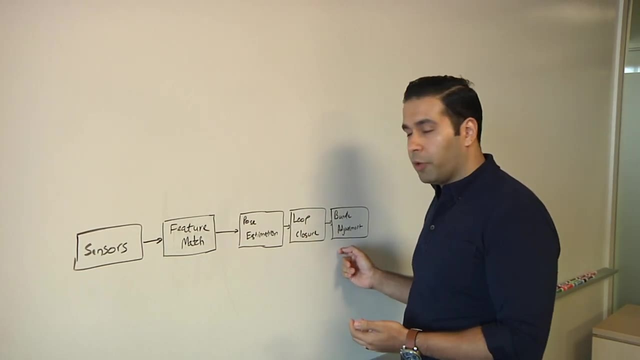 That further is used to come up with the basic odometry, visual odometry or pose estimation. And then you can do further refinements with loop closure and another stage following that called bundle adjustment. So let's drill down into each one of these. 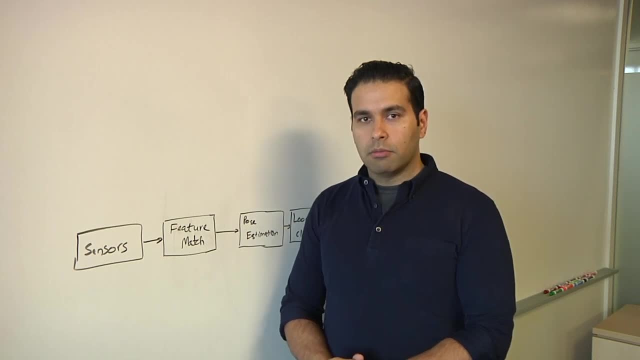 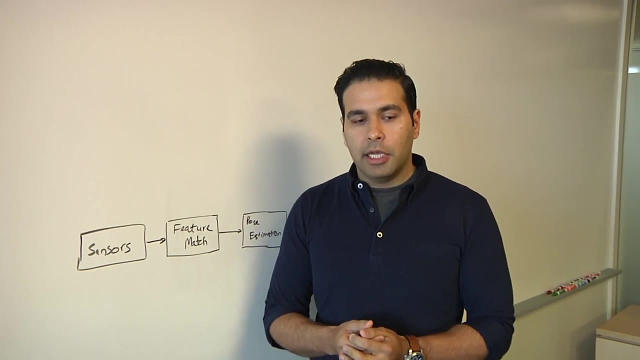 So what happens on the sensor side? What's actually going on in there? Sure Great question. So the sensors like over here, what we're talking about is, you know, SLAM. typically in a lot of the camera-based applications, they use some type of camera sensor as input. 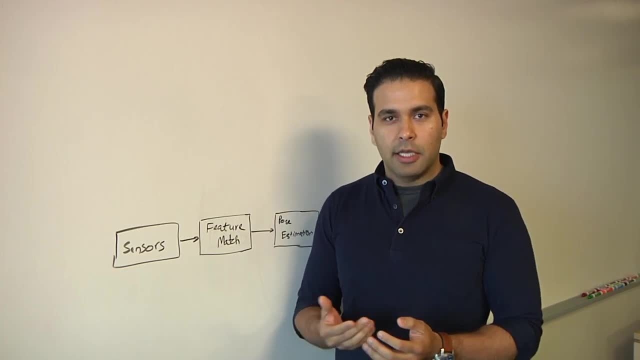 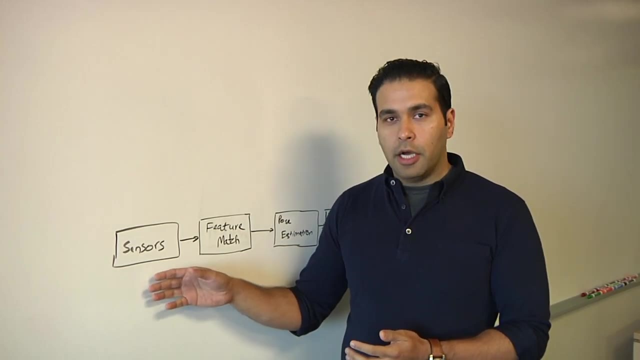 But you know, if you see the autonomous driving space, they use a lot of radars and lidars, So you know it's typically sensor agnostic. So from a sensor perspective, this could be RGB camera, grayscale, time of flight. 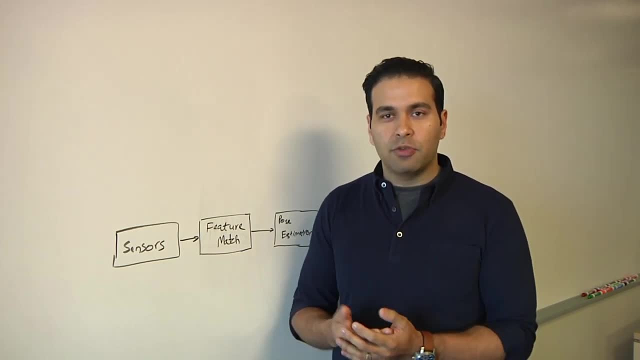 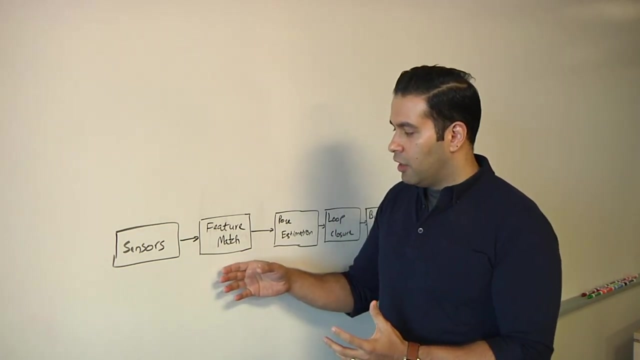 stereo could be radar, lidar. I've even seen some cases where customers use like a barometer. If you use the sensor properly for its particular capability, you can feed it in towards your SLAM block. So if you focus on visual SLAM, which is more camera-based in the feature extraction stage, 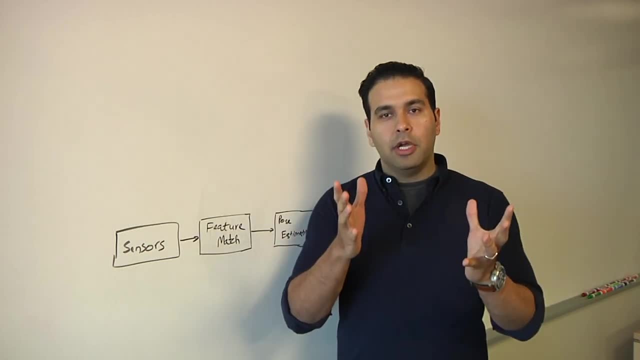 this is more or less how we perceive the scene. Like when we look outside the world, how do we understand the different points in the scene? Well, we look at corners, we look at edges, we look at colors and things like that. 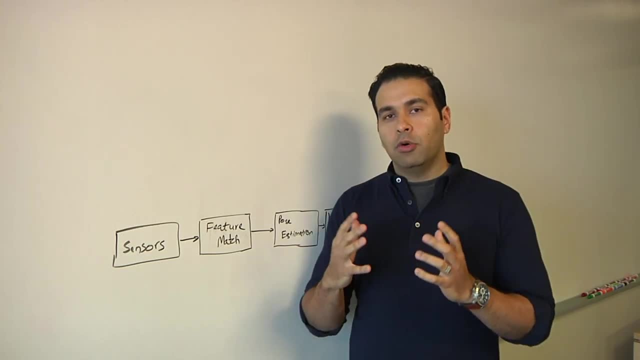 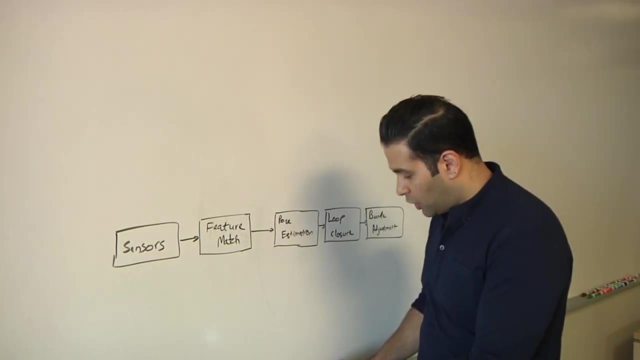 So we look at corners, we look at edges, we look at colors and things like that. So in the feature matching stage, the goal is basically to find these specific corners that may be there in a particular environment. So you can say that if a camera is looking at this duster over here, these could be several. 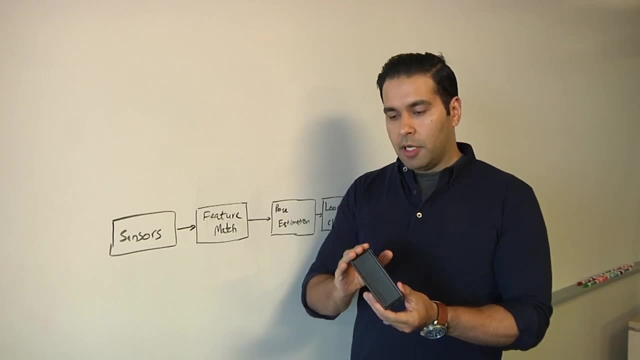 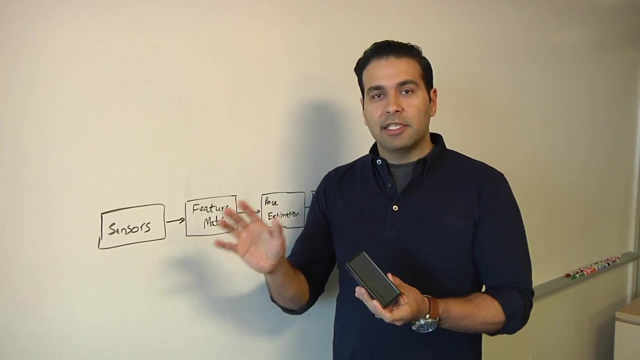 corners that are there on the duster. But when you move to frame number two, the goal is you want to be able to identify, you know, one, two, three, four as the same corner points or interesting points in the second frame. 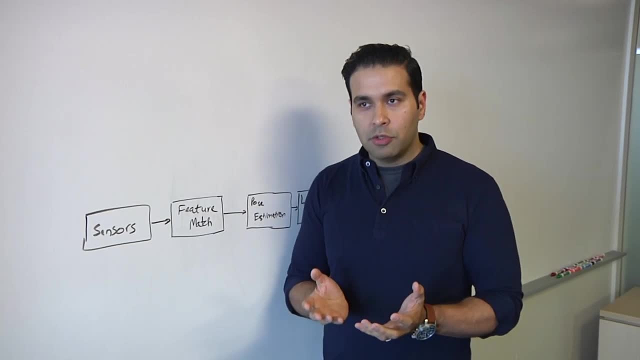 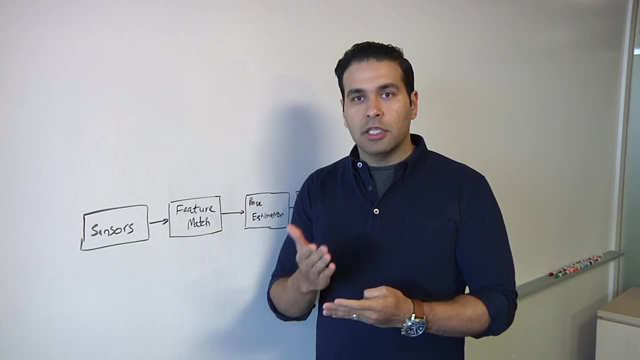 Now how you relate those two. There are a variety of algorithms that can be used to do that, but typically for feature extraction you can use things like SIFT, SURF, difference of Gaussian, ORB and things like that. 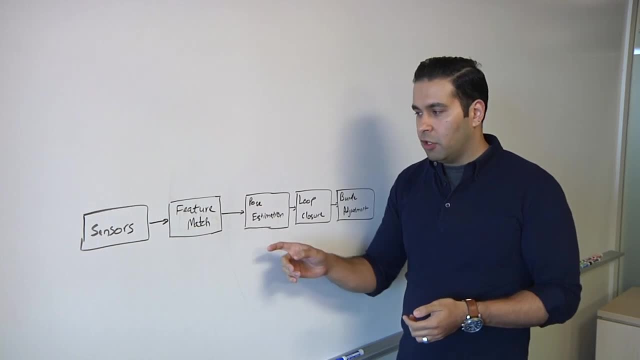 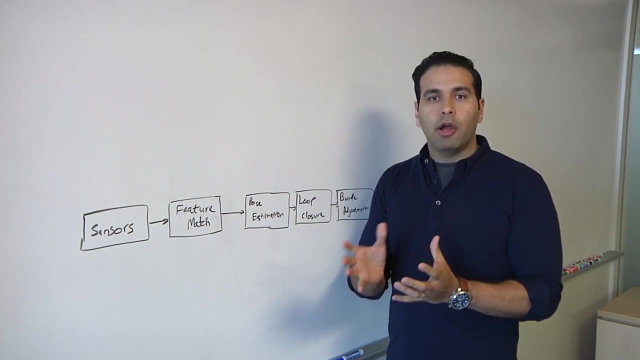 Moving now to the pose estimation stage, you take these features that you have found right over here and you identify how they move from one frame to the next. That allows you to estimate how the camera or the object has moved from one frame to the next. 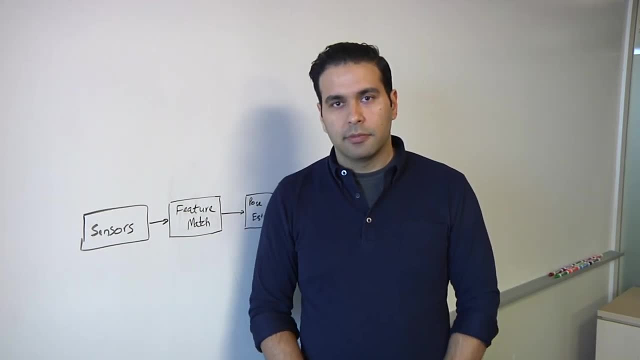 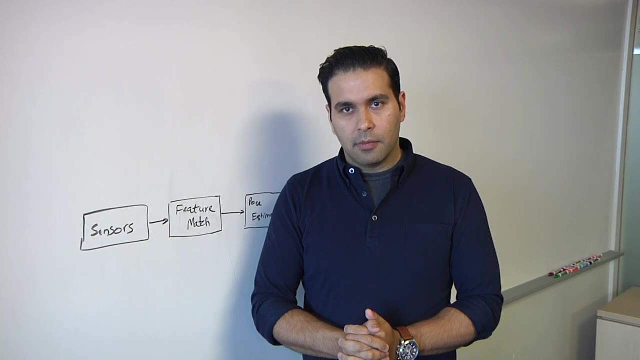 The human brain tends to pick this up very easily with object permanence. but if you're looking at a billboard In a car and the car has cameras on it and you're driving along, does it understand that this billboard is the same billboard in the next frame as what you saw before? because 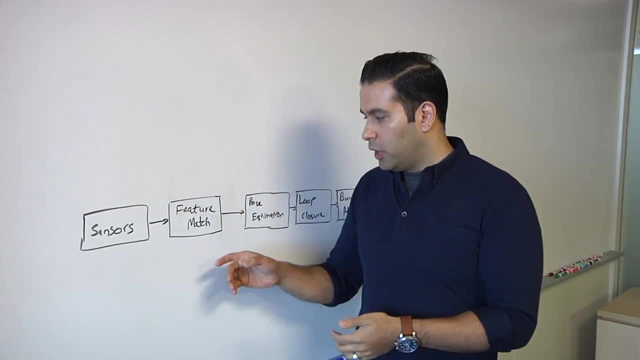 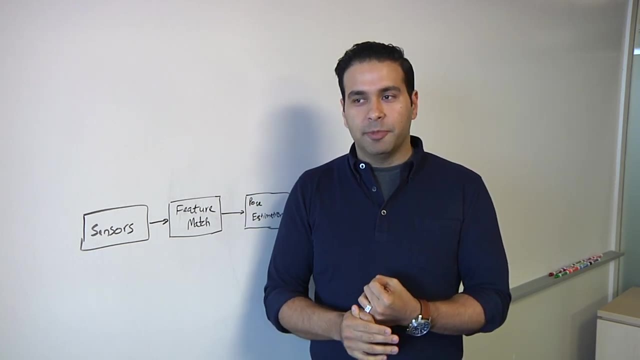 you're coming at it from a slightly different angle. Yeah, so that's a great question. So that's where your feature matching stage actually comes in, because the goal of you know the features like SIFT, which stands for Scale, Invariant, Feature, Transform or 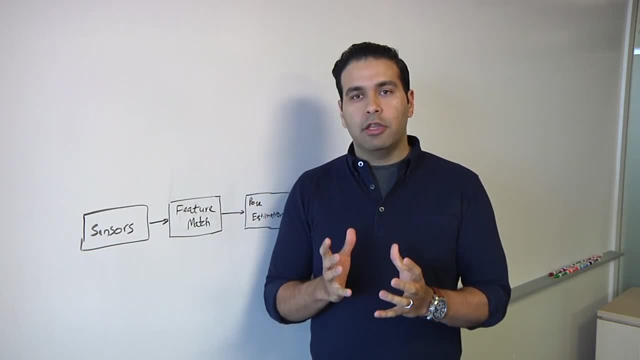 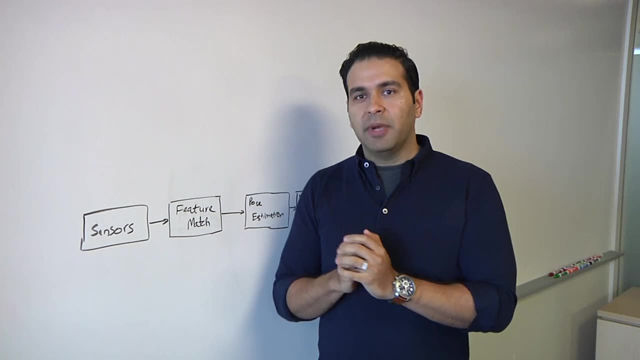 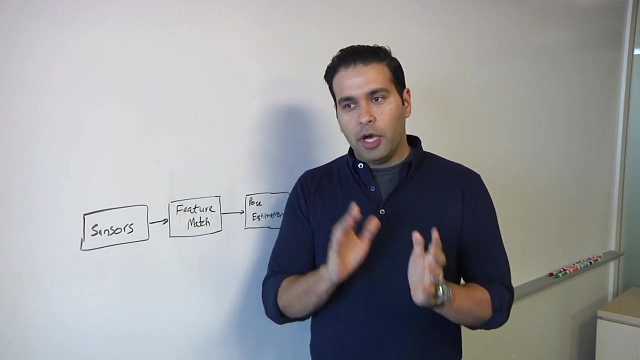 ORB descriptors and things like that. The goal is to identify those interesting points or corners in frame number one, and when you see that, When you see the same object in frame number two, these feature matching capabilities actually allow you to identify that. let's say, those four corners that you saw in frame one are 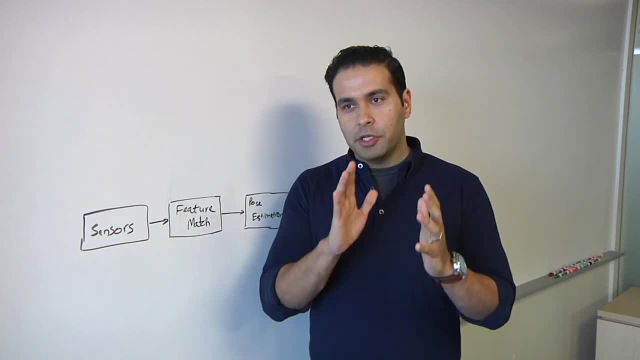 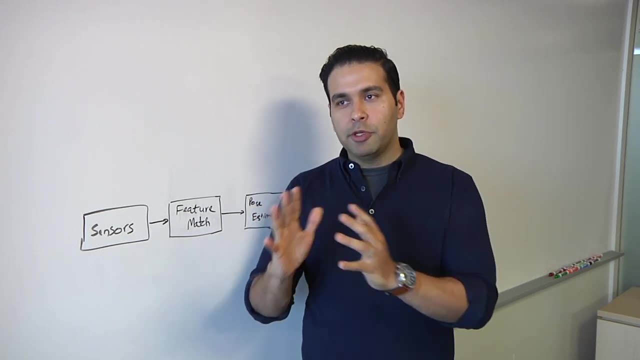 the same four corners that you see in frame two. Once you have that information you can essentially correlate those two frames and say, okay, it's moved so much from frame one to frame two. from that I can articulate and understand how my camera has moved in the scene. 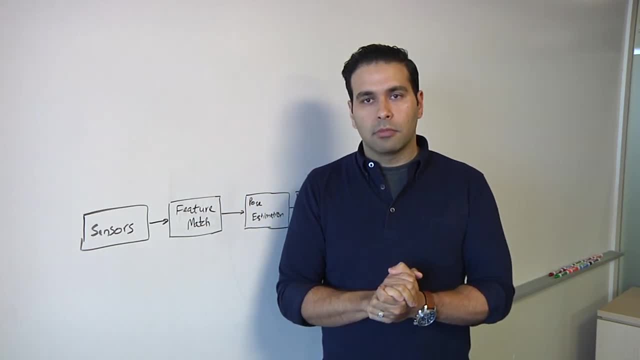 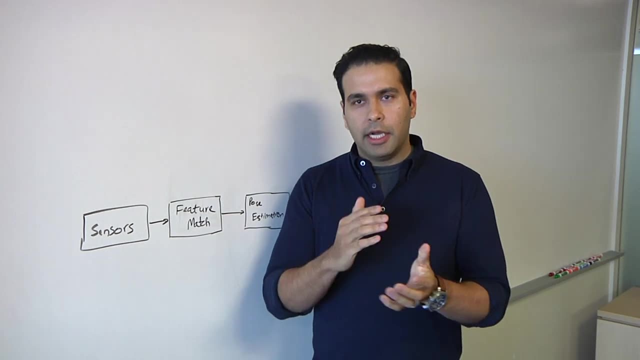 Are you working off of probabilities of this? is 99 percent probability that this is the same object that you were looking at before? Yeah, there is a variety of probabilities that come into play over here and you know the thresholds on that can be varied depending on you know the implementation. 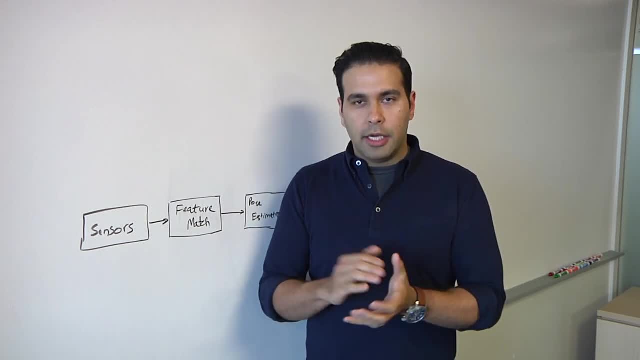 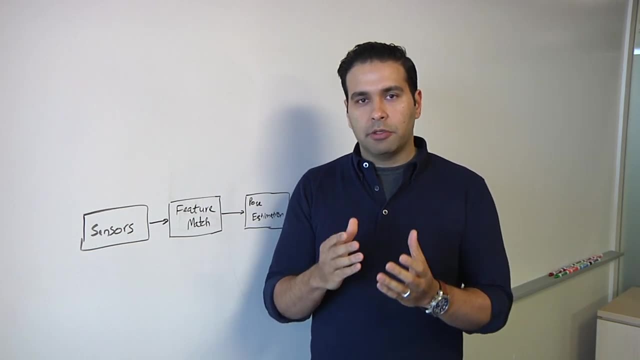 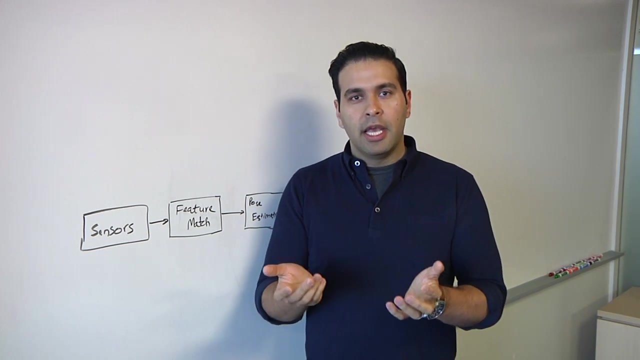 Everybody has their own flavor for the algorithm, so it varies from one case to another, But there's typically probabilities that there's also outlier illumination, because obviously there is noise that comes up when you are trying to match these feature points, and that's where you know techniques like RAN. 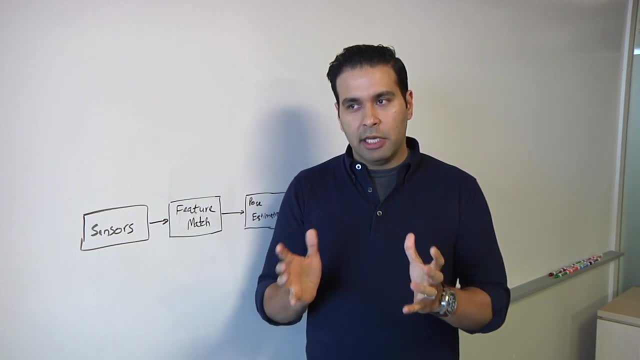 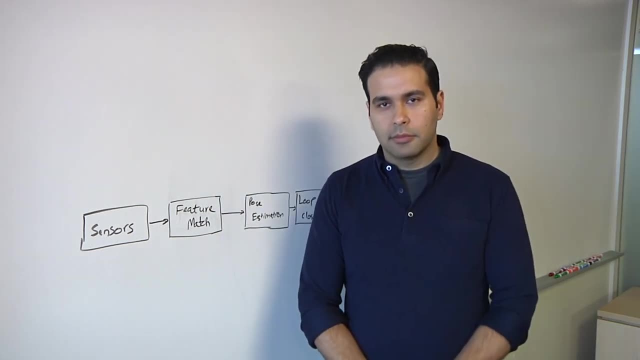 Yeah, RAN sac, which are used to eliminate outliers and keep predominantly the- you know, the key feature points that correspond well from one frame to the next. So what else is in the flow here? Okay, So once you have a pose estimation, you have the next step, which is called loop closure. 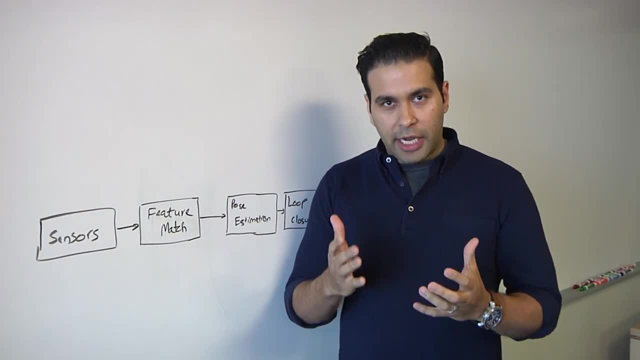 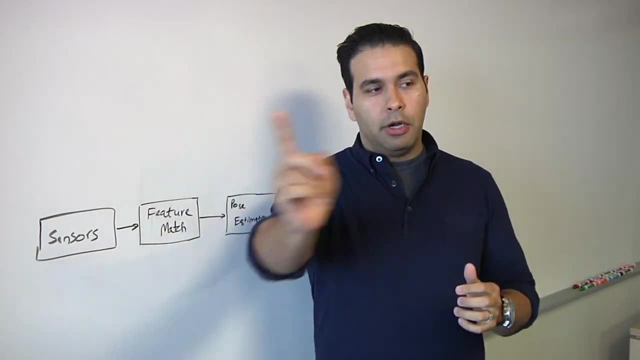 So the goal of a loop closure is basically to identify that you have visited or you have been to that particular spot before. So a simple example is: let's say I'm in this room over here, If I walk around this room and I come back to this particular point- 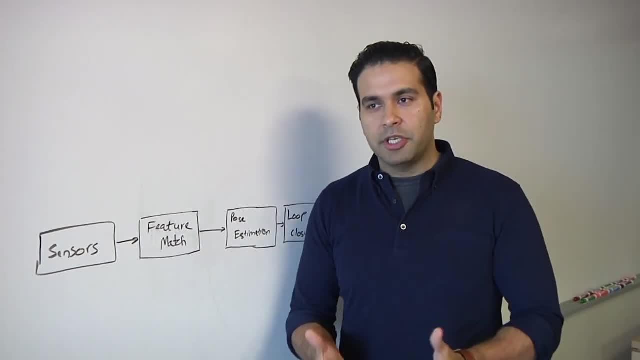 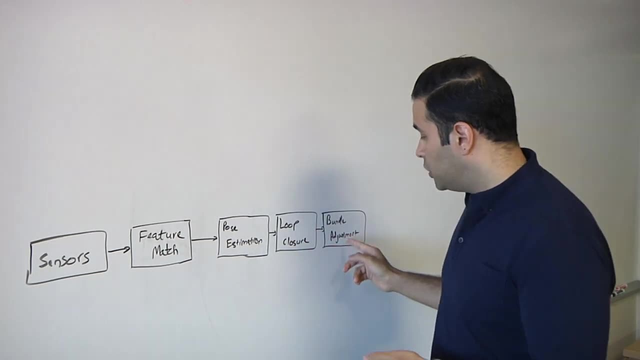 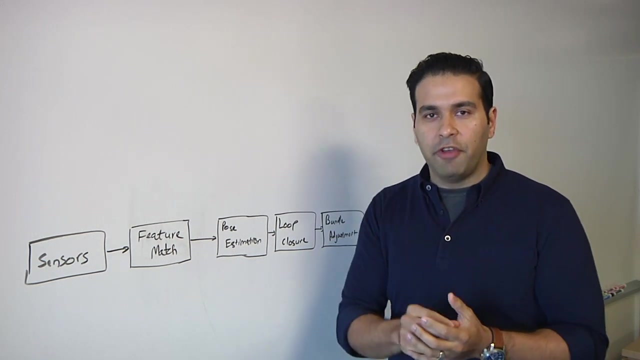 Loop closure would help me identify or establish that. hey, I have been over here before, So it's not a new area. that it has to determine And then bundle adjustment is a common step that is used to you know. further, refine the aggregation of errors once you do a loop closure. 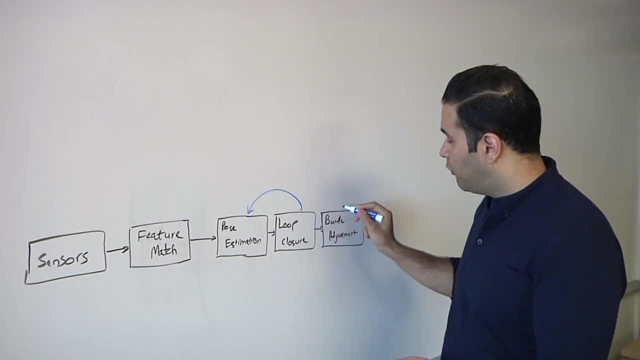 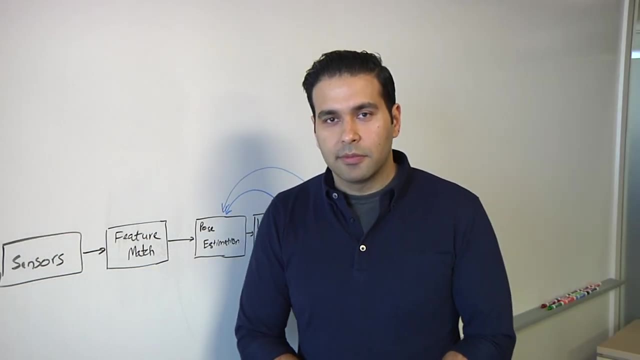 Now, typically, what you would see over here is a feedback step which would come from either loop closure or bundle adjustment coming to pose estimation. So what's that? Let's dig into this feedback a little bit more. What's actually going on here and what's the impact of this? 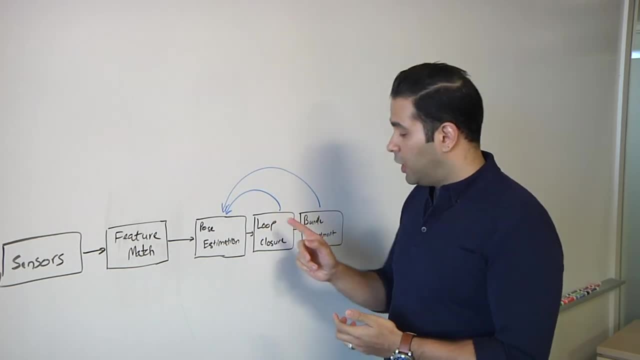 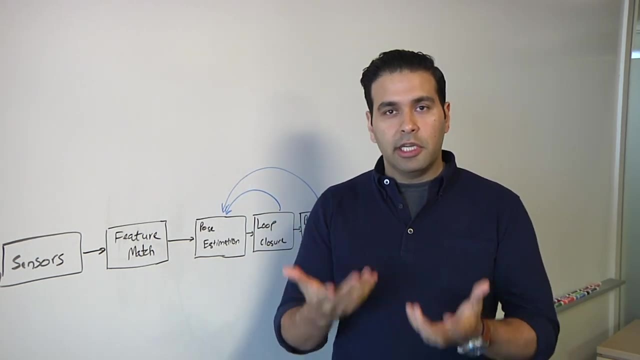 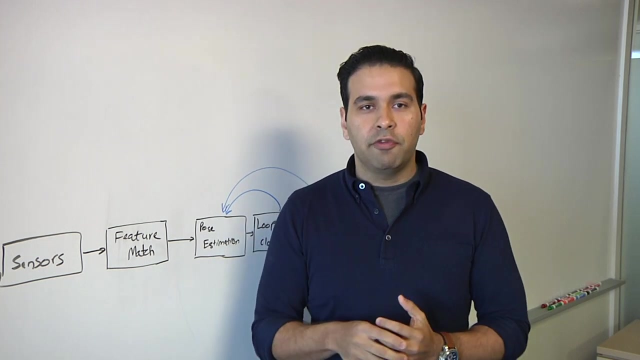 Sure. So, as you can see, basically loop closure and bundle adjustment, both feedback into pose estimation, because what happens with this feedback is you're constantly refining or updating your state estimate, which is basically your pose for your camera, based on the additional information that you have caught by, let's say, you know, walking around the scene and 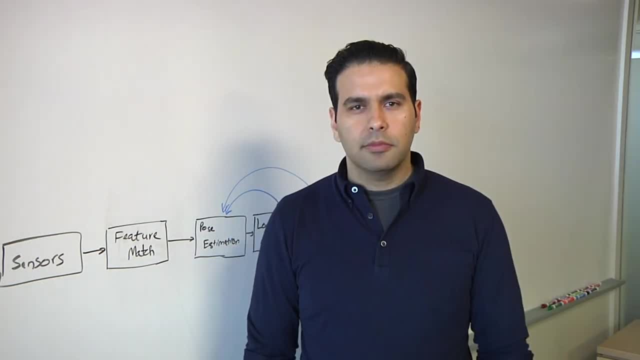 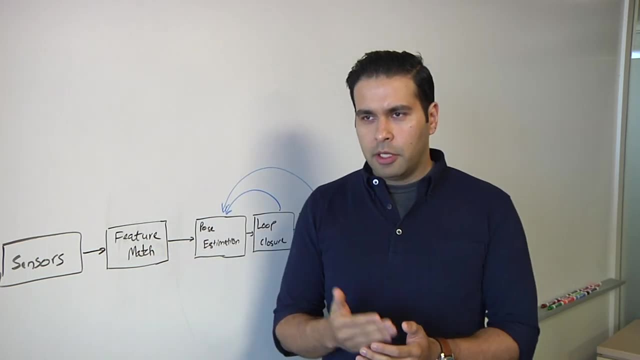 building a more accurate and a robust map. There's a couple of terms that tend to go with this, one of which is VIO. How does that play in here? What is that? Sure, So great question. So the terms that I think interchangeably used in the industry. there is visual odometry. 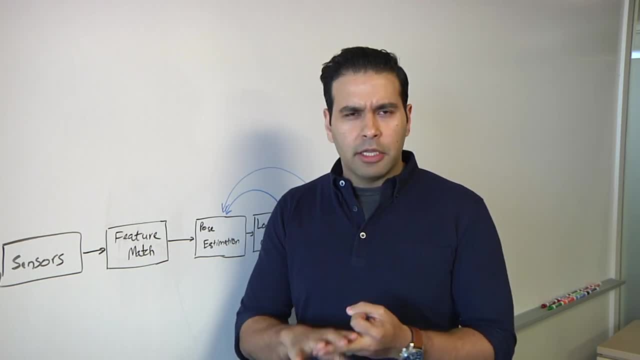 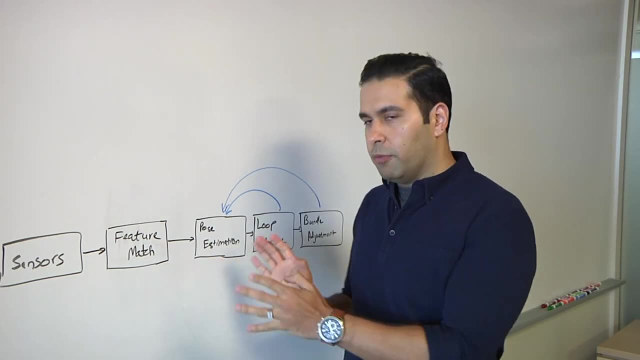 which is VO, or visual inertial odometry, VIO. There's also SLAM and 6DOF, which is six degrees of freedom. So visual odometry and VIO: they're somewhat similar in the sense that there's typically no feedback going from loop closure and bundle adjustment, as compared to SLAM. 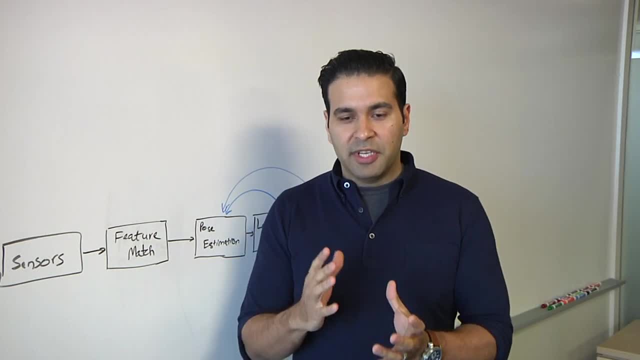 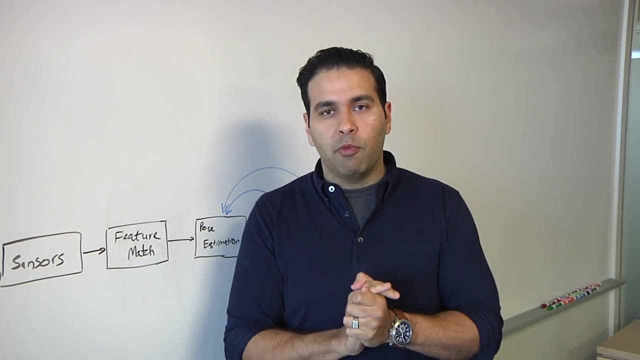 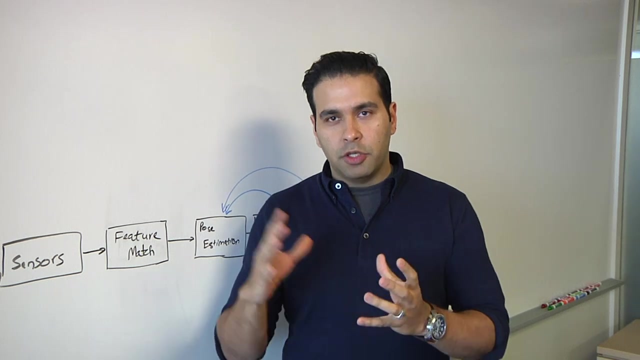 Okay, So visual odometry is more local problem in the sense that, okay, let's say I have frame one and frame two and I know how my camera- I'm just estimating how my camera- has moved from one frame to the next, So it's far more local versus SLAM uses a lot more global data because you're building. 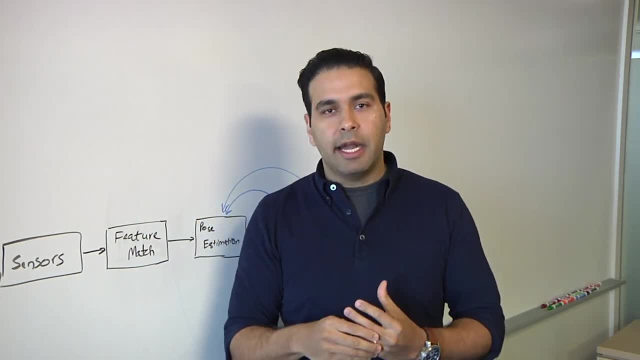 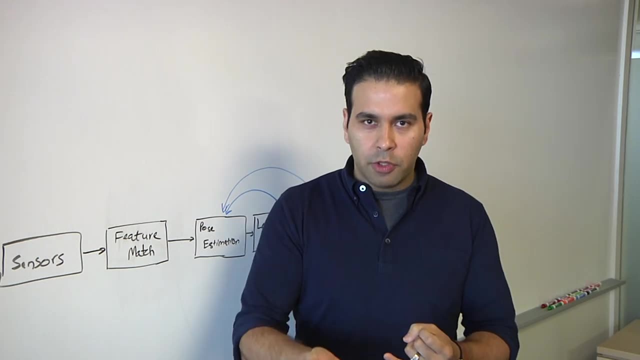 a map and as you are building more and more data in that map, you're getting a more accurate representation of your position. furthermore, updating your camera position over and over again with loop closure, relocalization and all those things. So it depends on the application, depends on the compute budget that your particular 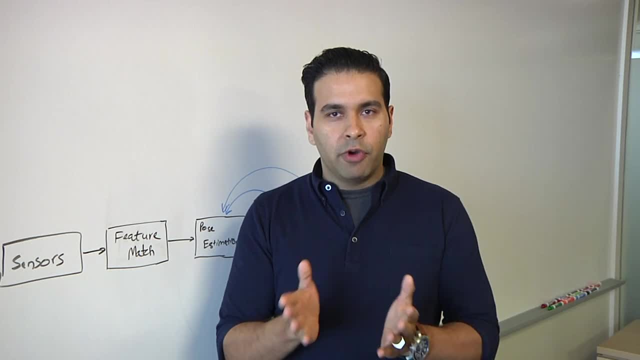 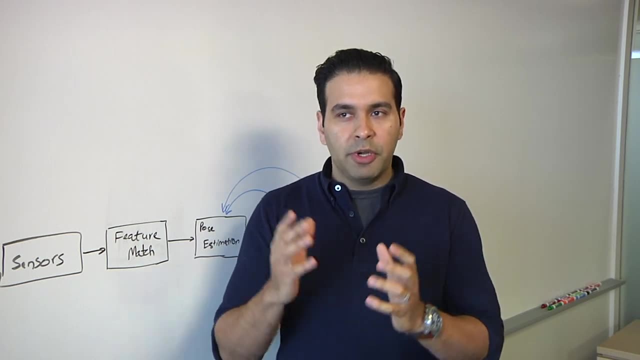 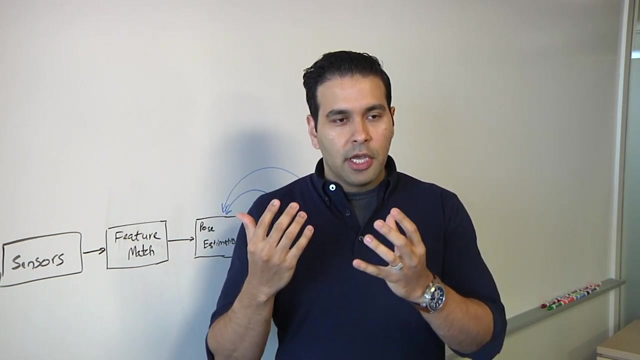 processor or your platform has and the varieties of applications are different. So, if you're talking about drones or something like that, I've seen many cases where they just use visual inertial odometry, because for them they have to build a very large map and having that much data to keep locally is not possible versus on mobile phones or 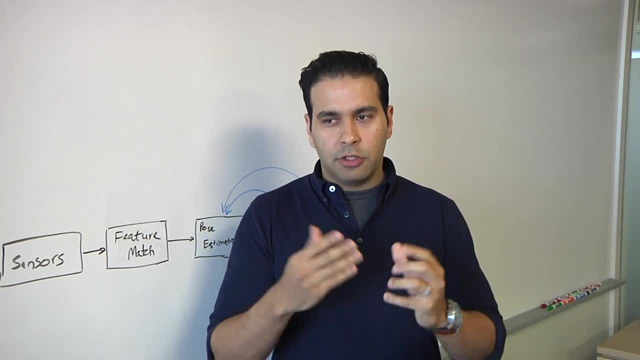 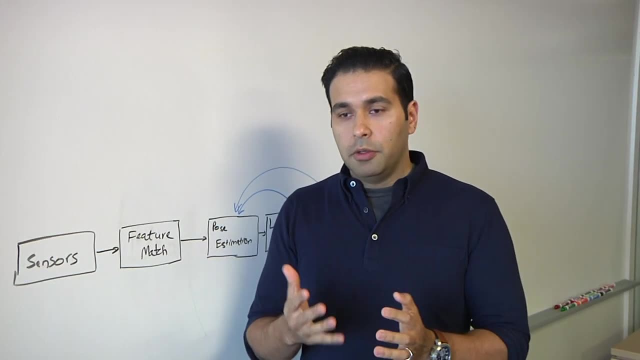 where you're doing augmented reality, it's usually a lot more smaller playing area, So SLAM is a lot of times more applicable over there. Okay, Like all electronics, something always goes wrong. What can go wrong here? So with SLAM or with VIO, typically it comes to whatever are the limitations of your sensor. 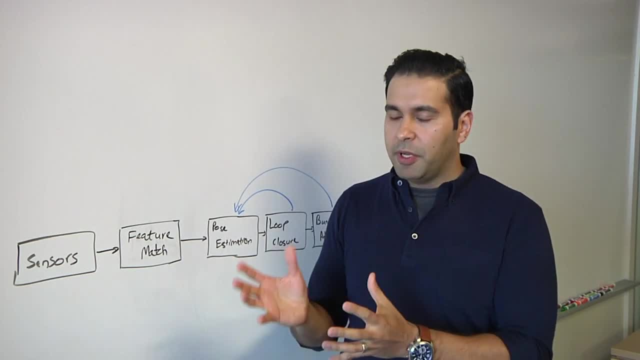 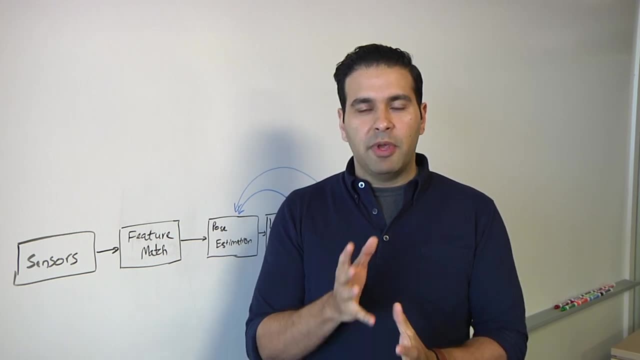 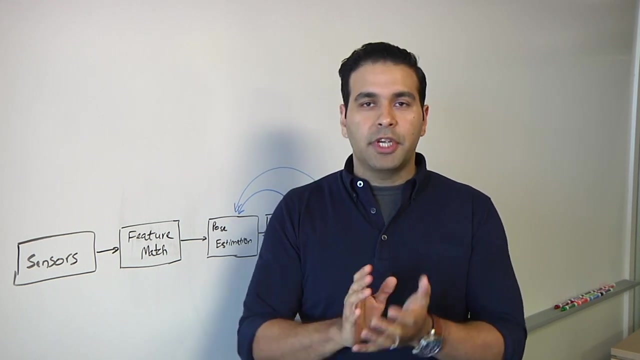 So in SLAM, for example, they typically do a combination of a variety of sensors, So sensor fusion. most common solutions typically have maybe a camera along with an IMU, which is an inertial measurement unit, allows you to understand how your object is more or less. 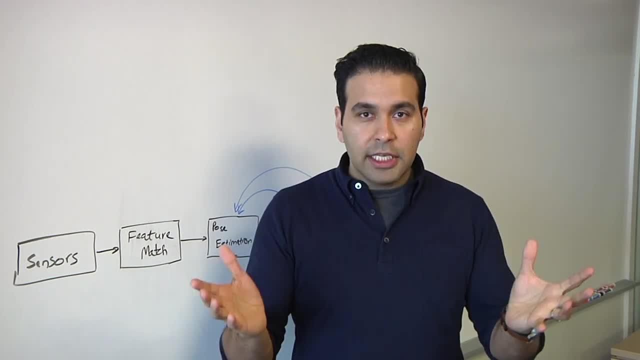 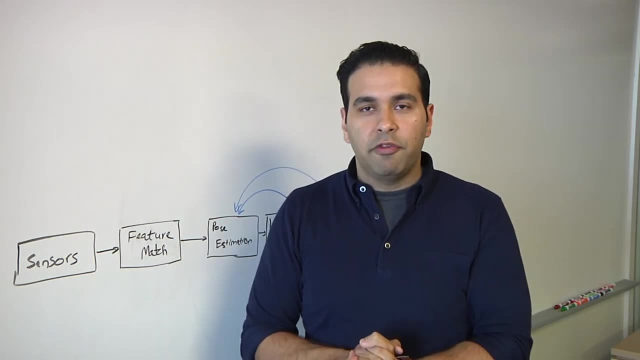 rotating in the scene. Now cameras also. although they can see the world very easily, there are some cases where there are limitations. If your camera is looking at a flat wall like this, well, there are not many features over here and if you were to just move the camera around looking at a flat wall, SLAM wouldn't. 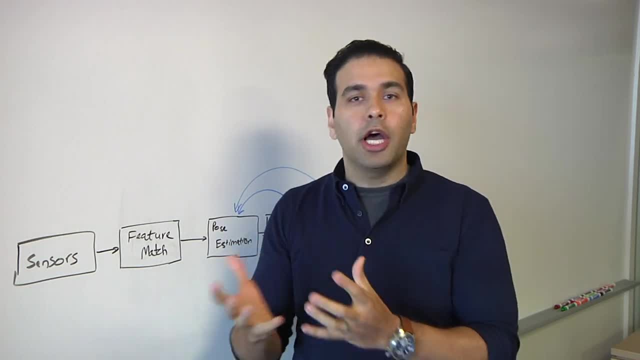 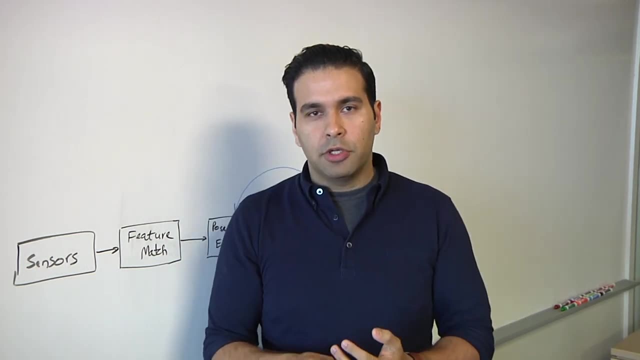 really be able to work too well, because just using visual data you don't know how the camera is moving. Other than that, also, there are noise models that you have to estimate very well. So typically for your IMU, you have to understand the different types of noises that are there. 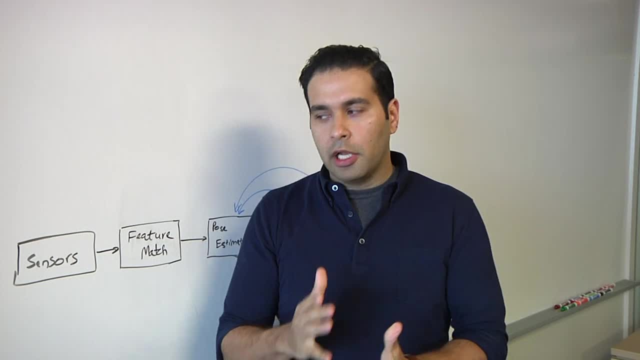 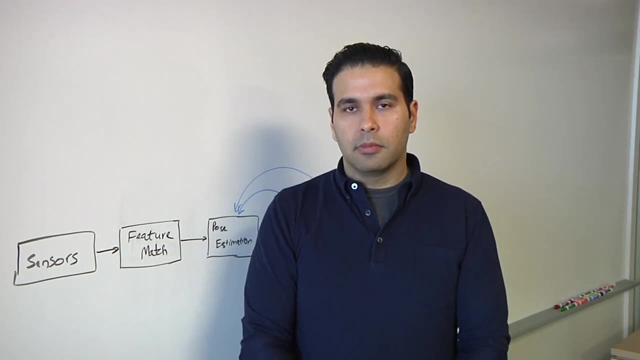 on the particular device and be able to accurately model it to further give you a much better SLAM implementation, And sensors also need to be recalibrated over time because they do begin to drift. What you start out with is not necessarily what you end up with. 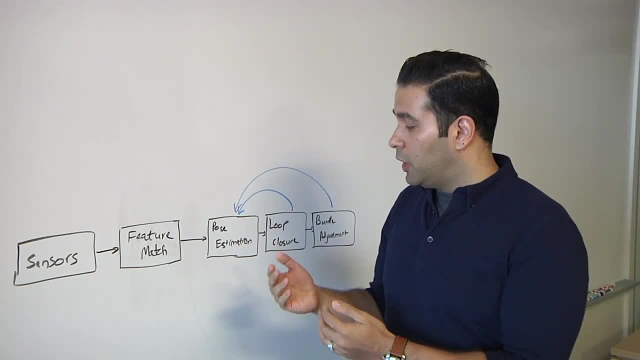 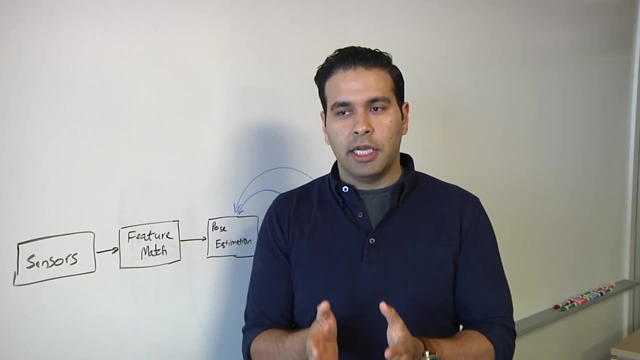 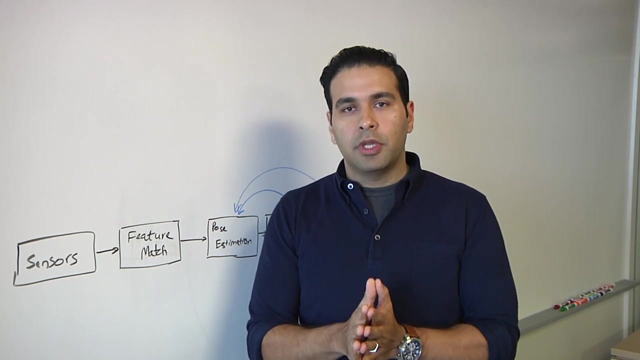 How does that affect this? Yeah, so I think. typically with SLAM, for example, with loop closure, and having relocalization, which is understanding relocalization with loop closure. to understand that you have come back to your original point. that helps with a lot of cases of drift. 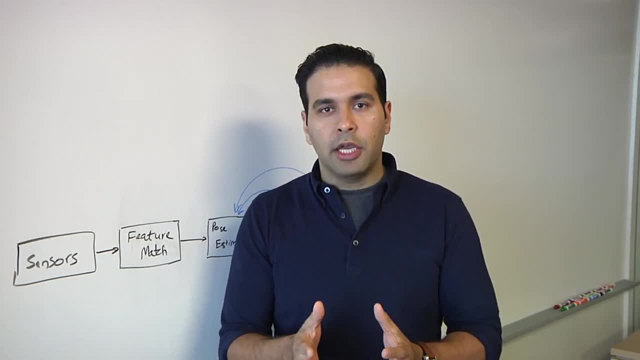 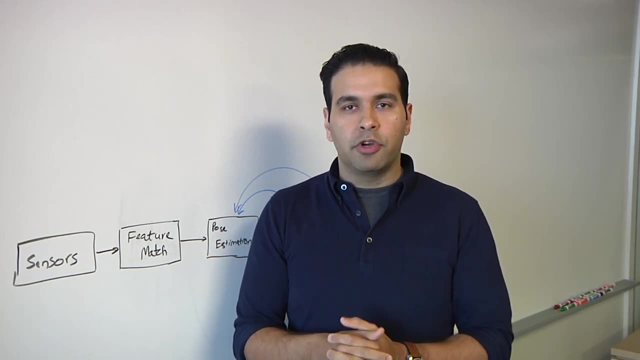 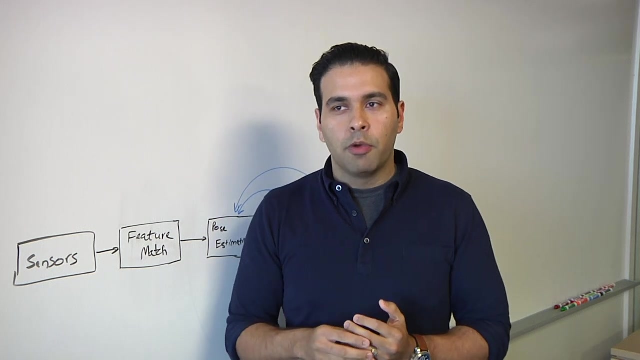 If you did not have this and were pretty much just relying on, say, for example, your visual inertial odometry. in those cases, you could probably expect a lot of drift to happen, unless you have an algorithm or an implementation which is very, very accurate and is not prone. 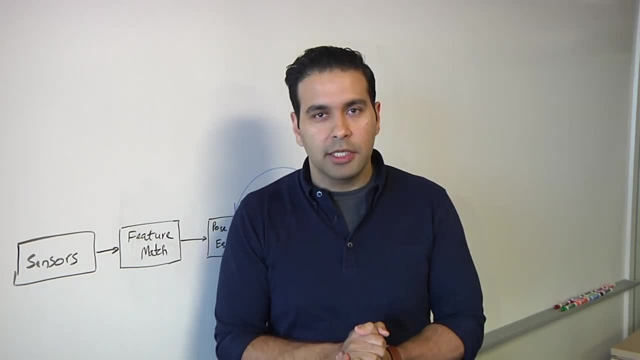 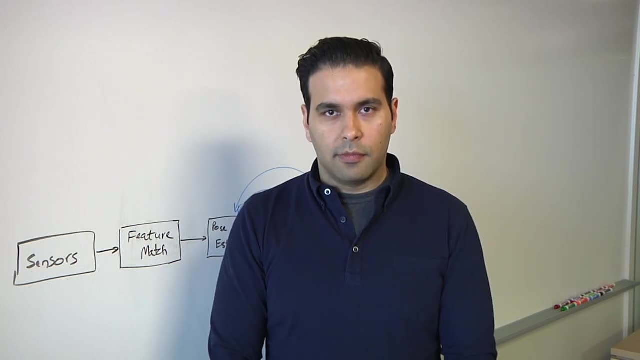 to any noise, which in most cases, it probably is not going to be the case. Another angle on this is the power and performance Which obviously you need as much performance as you can possibly get and you need as low power as you can possibly get. 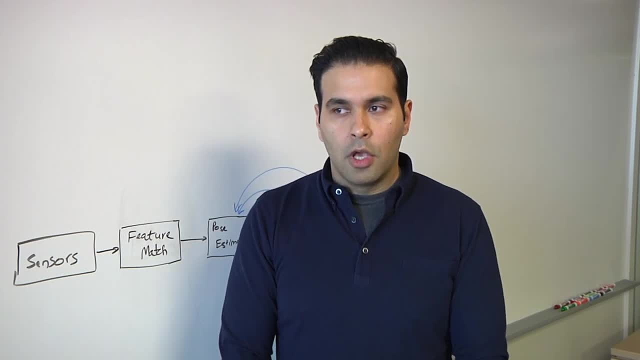 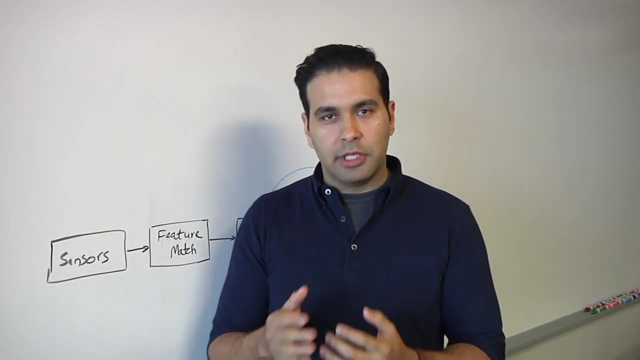 What can you do here to actually reduce the amount of power and improve the performance? Great question. So SLAM as a technology by itself has been around for a long time, I think introduced back in the 90s, And you started seeing some real-time implementations coming somewhere in the mid-2000s, like the 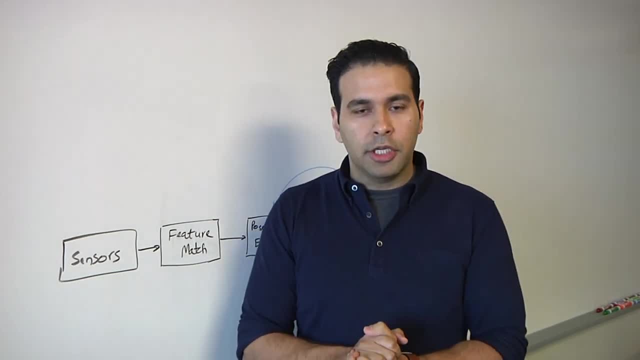 DARPA, Grand Challenge and Urban Challenge. Those contests were primarily relying on a lot of SLAM implementation. Yeah, So SLAM implemented a lot of SLAM implementations, but at that time you had rack-mount servers that were mounted in the trucks. You can't really go into production with something like that. So over years the algorithm has refined. It's gotten more power, efficient. Even our hardware has obviously improved. So you have seen implementations going on to CPUs, to GPUs and now even on mobile phones. 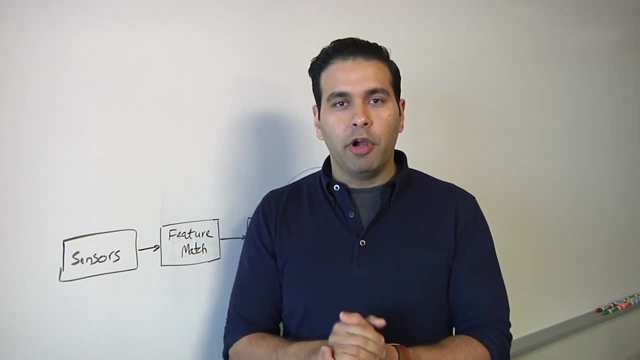 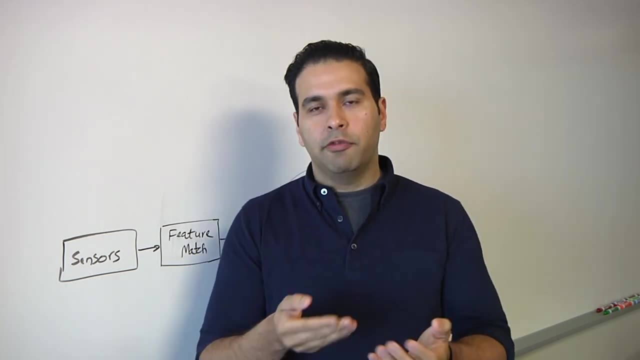 But power and performance are two things that obviously are very important for a customer, because you don't want to have SLAM running on a phone that you can run for 10 minutes and it gets super hot and then you have to charge it. 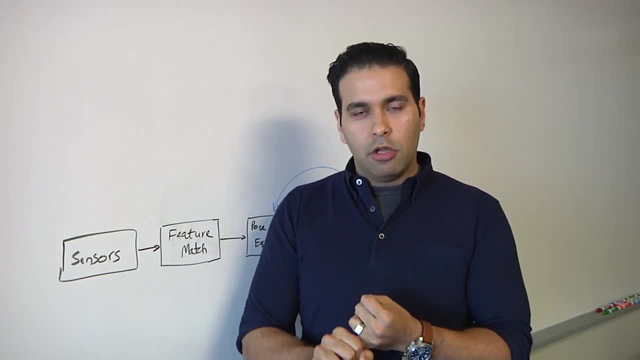 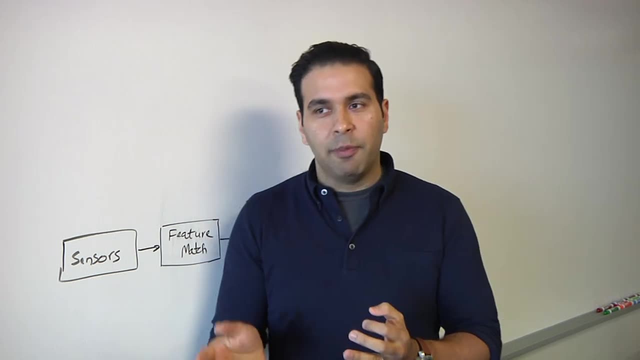 So power efficiency is very, very important. So, although the solutions run very well on CPUs and GPUs, obviously those type of platforms aren't built for these specific applications. So they work well, but they are power-hungry and not the most efficient. 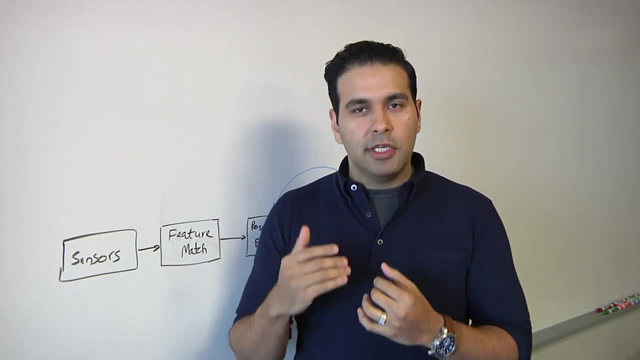 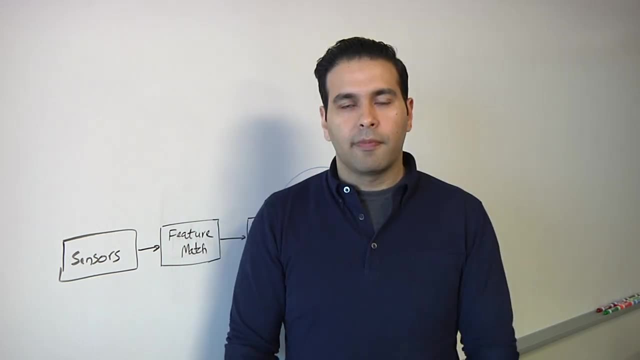 If you start scaling more towards things like DSPs or accelerators, you'll probably get a much better performance as well as a much smaller power envelope. Alongside of that, what's the next step? Outside of all this, there's been a huge push into accelerators on almost everything. 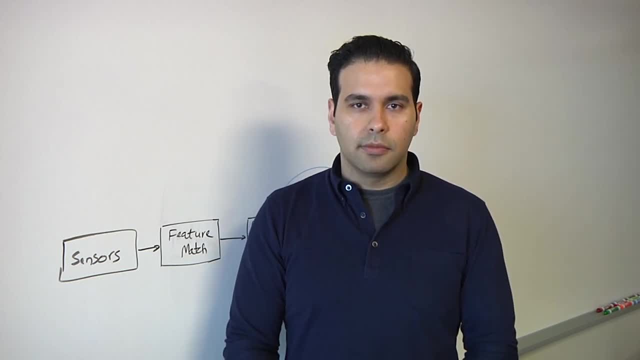 involving large amounts of data, which is what's going on here. What's the best platform for this? Do you stay on a CPU, a GPU, a DSP? Do you add accelerators in here? How do you make that choice? Sure. 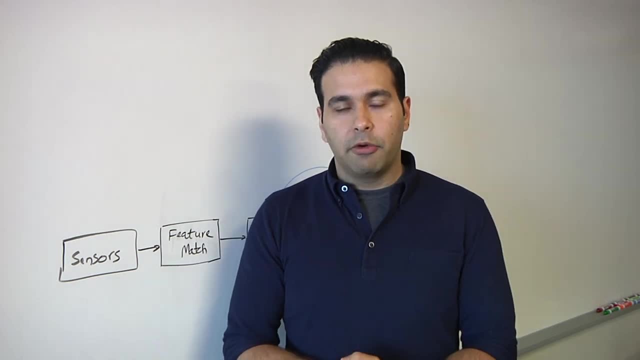 Great question. So I think DSPs is probably a great way to go right now. So CPUs are great for prototyping. in my opinion, You want to get some more performance or some more juice out of it. I think GPU is a good way to go. 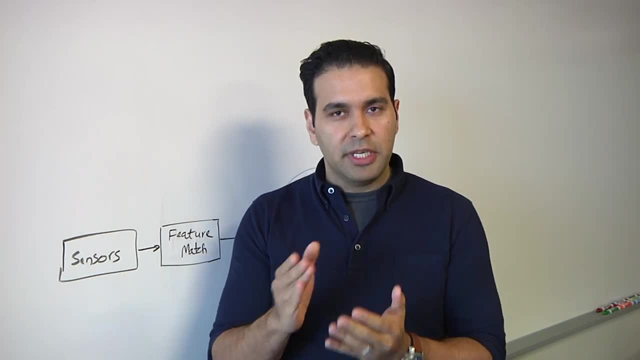 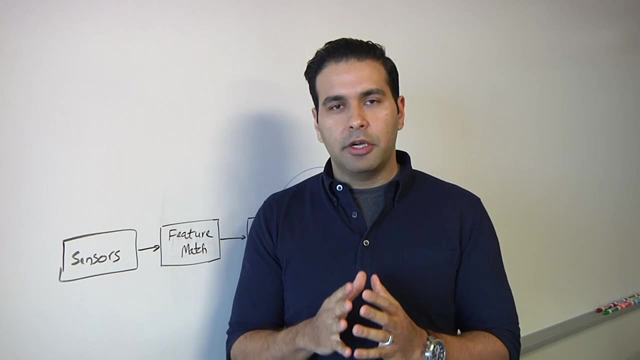 Once you start targeting large volume deployments, DSPs are definitely a great way to go. Hardware accelerator: I think it's still too early for SLAM, because hardware accelerators is typically some type of an RTL block which will give you a performance boost.